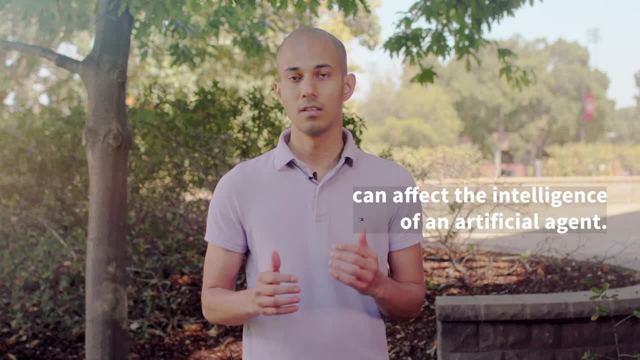 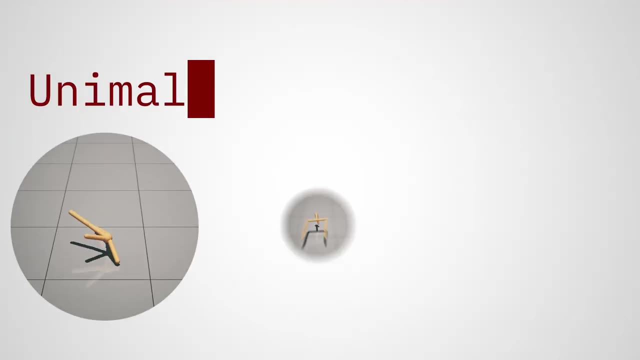 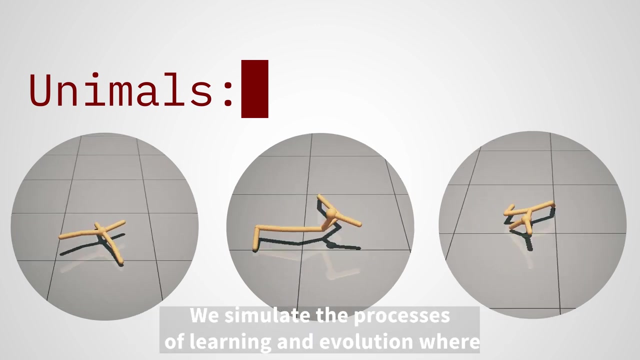 how evolutionary environment and morphology of an agent can affect the intelligence of an artificial agent. Inspired by nature, we created arthropod-like agents called unimals, which undergo mutations and natural selection in different environments. We simulate the processes of learning and evolution, where hundreds of these unimals learn to control their body to survive in their environment by 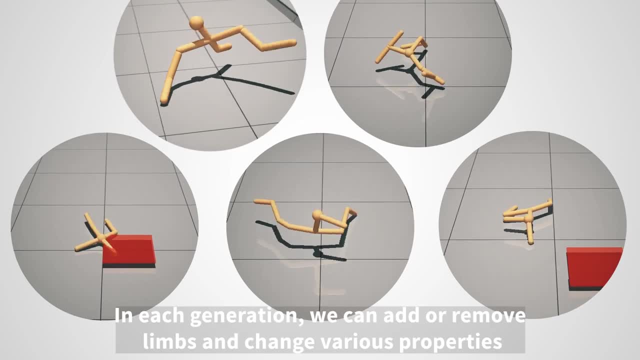 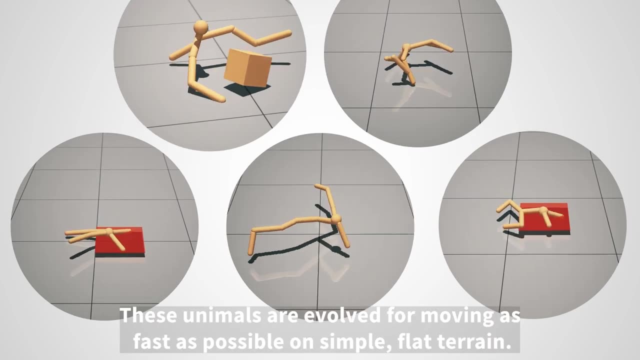 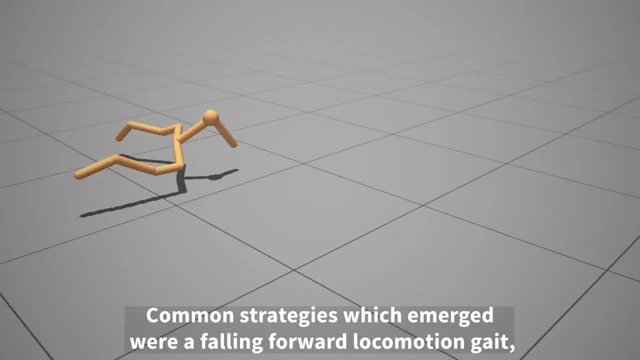 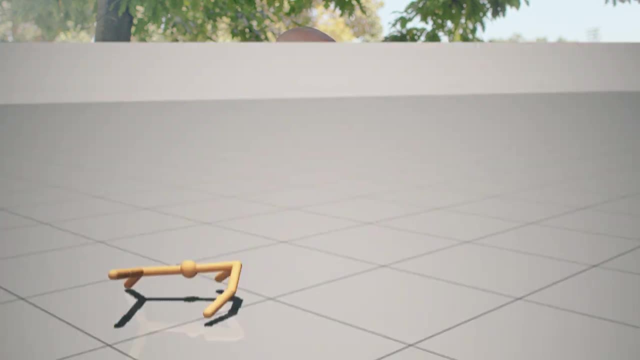 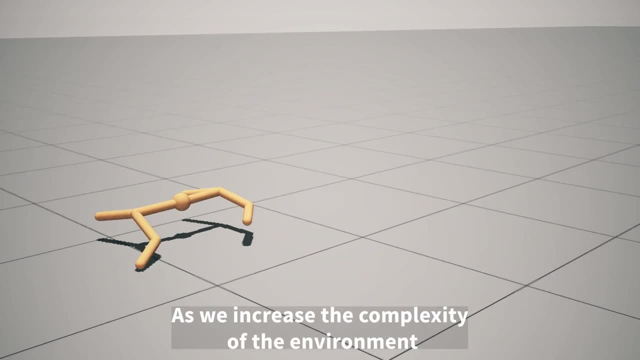 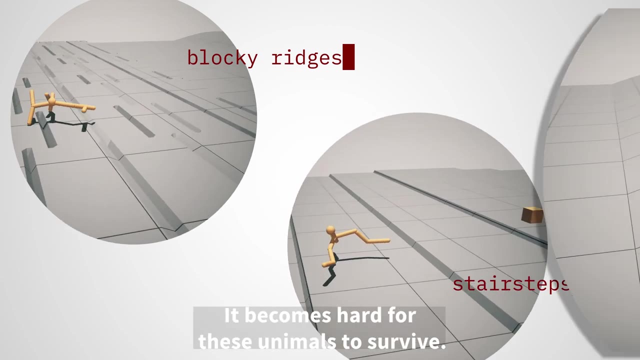 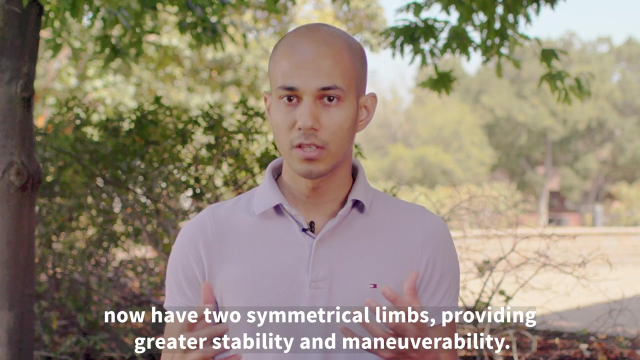 Another strategy was the emergence of a lizard-like gate. As we increase the complexity of the environment to include blocky ridges, stair steps and smooth hills, it becomes hard for these animals to survive. Instead of having a single limb attached to the head, animals now have two symmetrical. 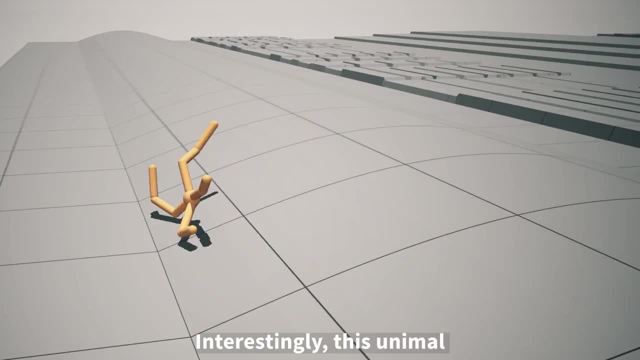 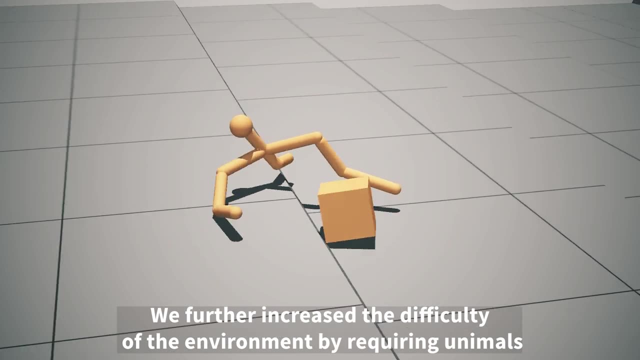 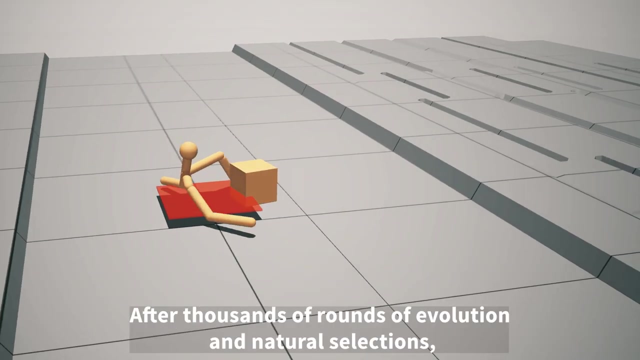 limbs, providing greater stability and maneuverability. Interestingly, this animal developed a locomotion strategy akin to an octopus walking on land. We further increased the difficulty of the environment by requiring animals to move a box to a target location in this challenging terrain. After thousands of rounds of evolution and natural selections, animals developed forward. 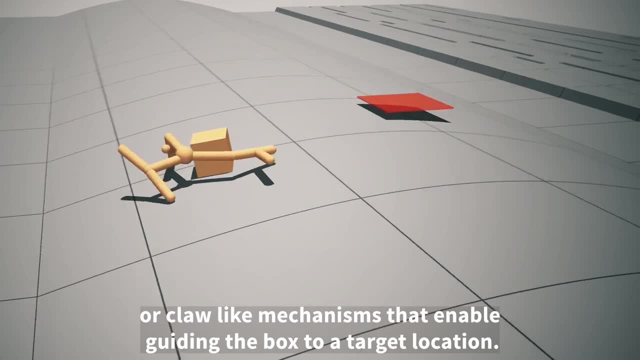 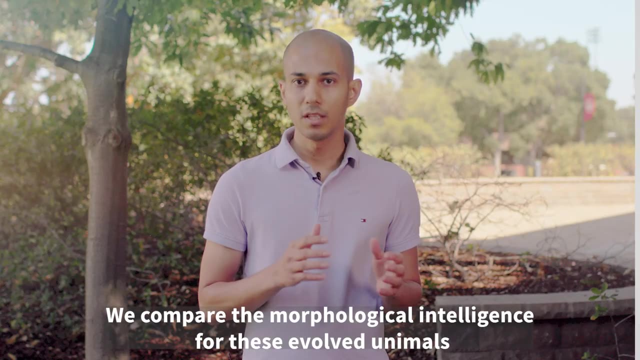 reaching arms, mimicking pincer or claw-like mechanisms that enable guiding the box to a target location. So are all these animals stable? Are all these animals equally smart? We compare the morphological intelligence for these evolved animals by measuring their ability to learn new tasks. 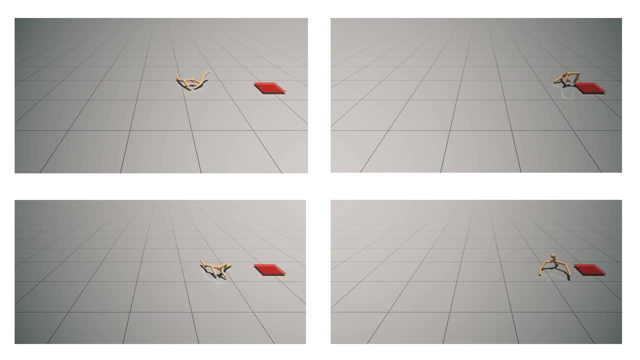 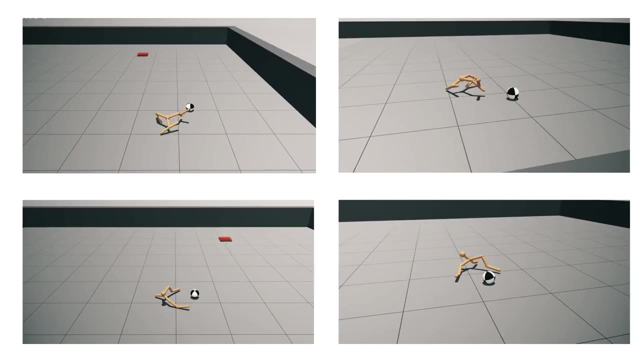 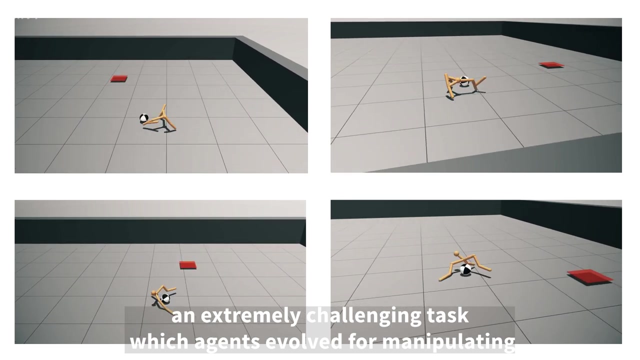 In this task, the agents have to patrol between two points. We find that agents that evolved in harder environments were more agile and could quickly change directions. Here the agents have to move the ball to a target location, an extremely challenging task which agents evolved for manipulating boxes could handle easily due to their evolved 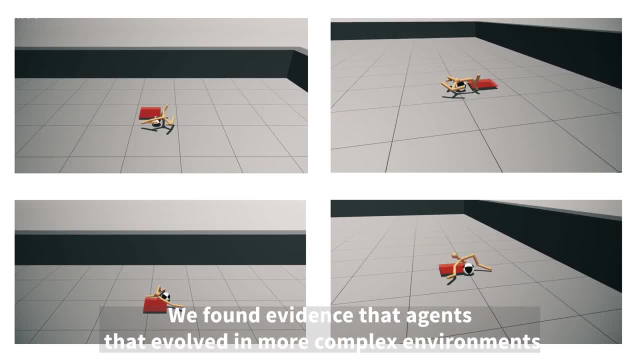 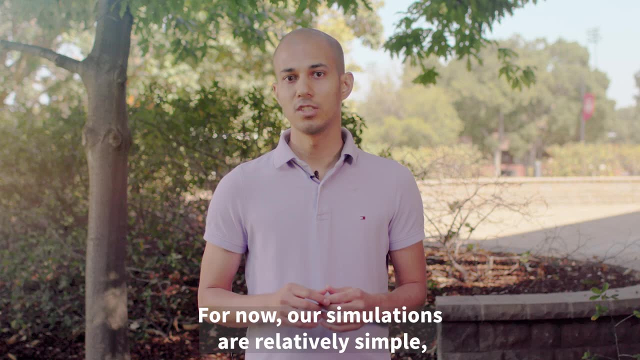 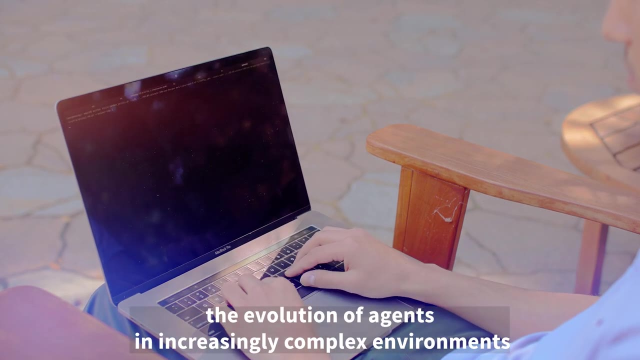 arms. We found evidence that agents that evolved in more complex environments got progressively better at learning new tasks faster and better. For now, our simulations are relatively simple, but we hope that with advances in computation and simulation capabilities, the evolution of agents in increasingly complex environments